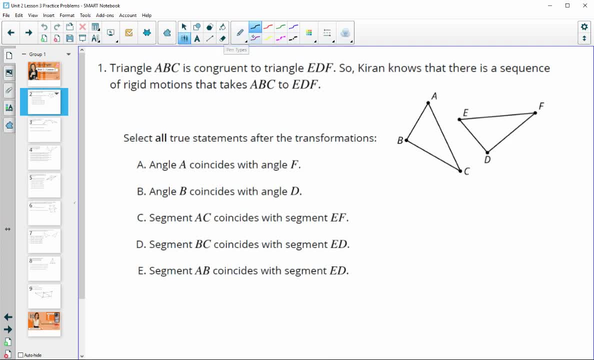 true statements after they do the transformation. So after the transformation is completed, would A coincide with F? And you can look in the statement here of which two triangles they say are congruent. So A is in the first spot, F is in the third spot. so those do not coincide. 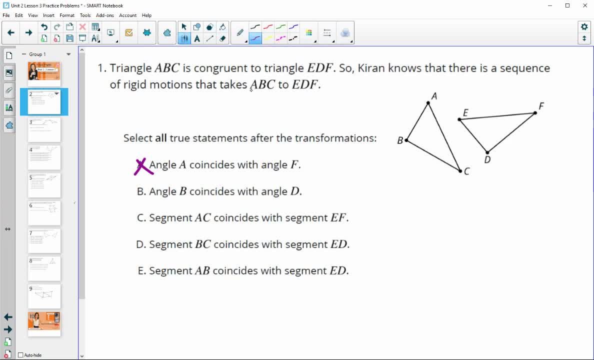 So that's one way you can actually just look in the statement. You could mark up the picture if you wanted. So, based on this statement, so A is going to go to E, so I could just mark that here as congruent. B is going to go to E, so I could just mark that here as congruent. 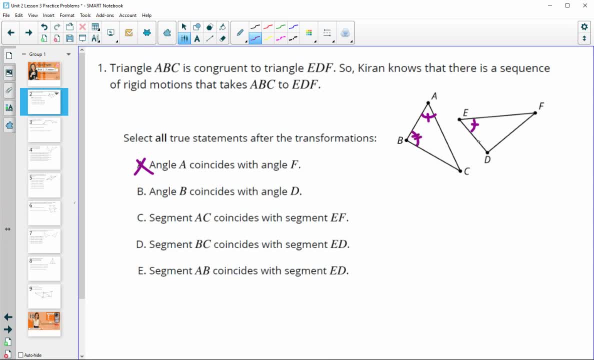 B is going to go to E. so I could just mark that here as congruent: A is the middle and D is the middle, so B and D And then C would go to F. So you could have them marked up like that if you wanted. And then it says A goes to F. 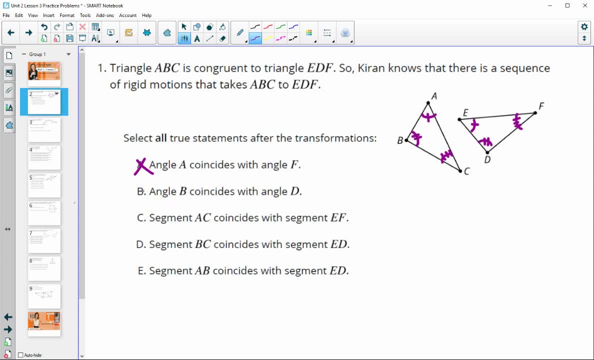 and that's not true. B goes to D is true. Segment AC coincides with EF, so AC and EF. So now you would check that those two angles are kind of the same. So this goes: AC is the one tick to three tick angle, EF is the one tick to three tick, so those do coincide. If you're looking at the 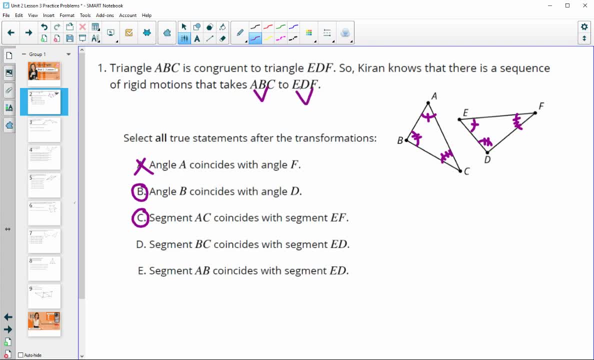 statement. you would see A and C are on the outer parts of the statement, so are E and F, so they would coincide that way as well. You can also even write this below: So EDF, and just check: A, C, E, F- They kind of land on top of each other. Does BC coincide with ED? So BC with ED. 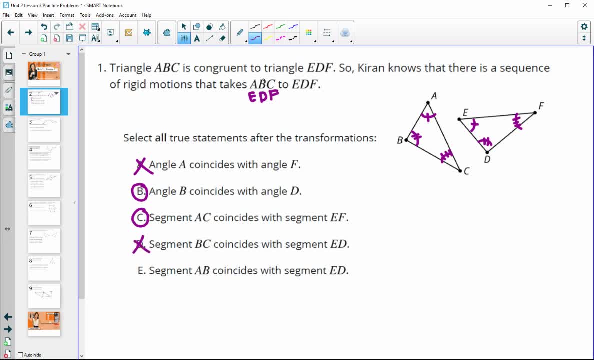 no, From the picture you can see that. You can see that from this statement here. Here's BC in the last two places and then ED is in the first two, And then AB coincides with whoops, AB coincides with ED. So AB is the first two slots, ED is the first two slots. So this would 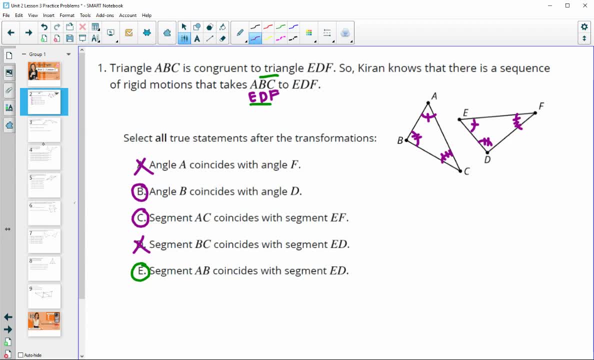 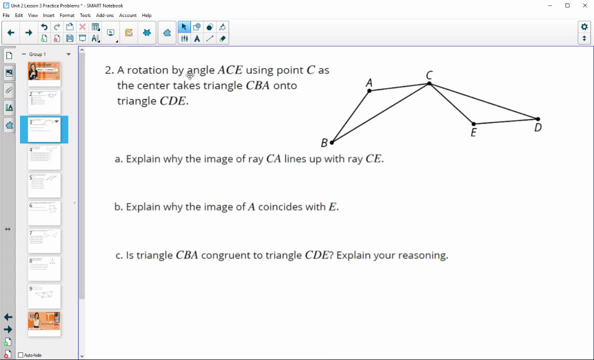 be true, All right. then at number two, it says a rotation by angle ACE. So let's look at that angle here. So rotation by angle ACE, Using C as the center point. So here's that angle. Takes triangle CBA onto CDE, So takes triangle. 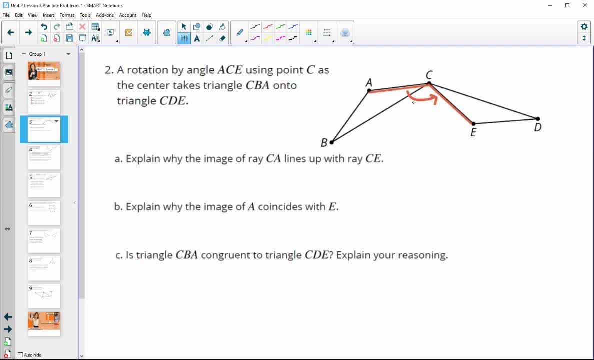 CBA onto CDE by this angle rotation. Explain why the image of ray CA. So why would this ray so CA? why would that ray? So why would ray CA line up with ray CE? And you can see that those rays are created by this angle or they're kind of the same angle as that angle, ACE. So this is. 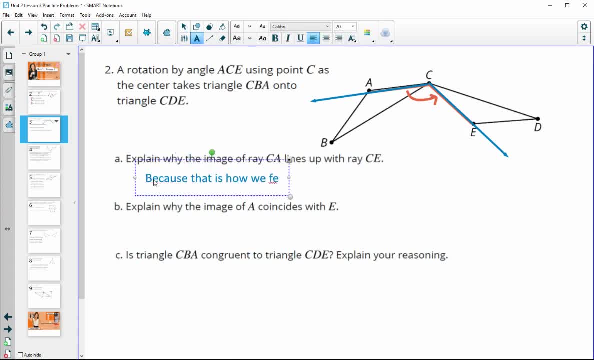 because that is how we define the angle. So this is because that is how we define the angle. So this is because that is how we define the angle. So this is because that is how we define our rotation. So we said to rotate it by angle ACE, So that side AC or ray CA would rotate over to 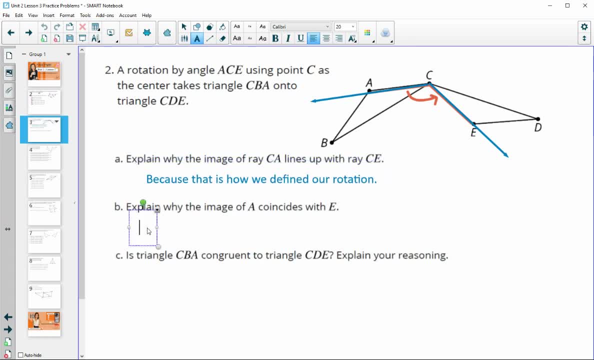 ray CE. So we defined it like that. So explain why A will land on E. And so we know that these two triangles are congruent to each other because it's saying that it will take triangle CBA onto CDE. So we know that these two triangles are congruent to each other because it's saying that it will take. 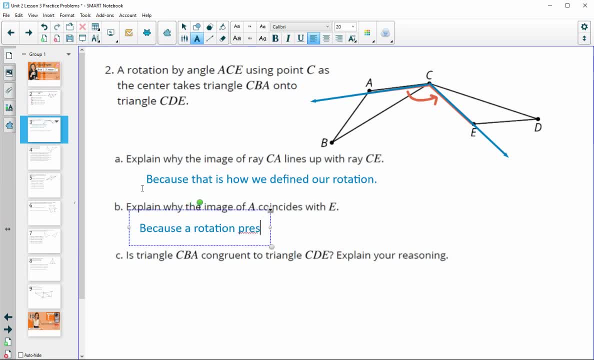 triangle CE to that side and then that side ACE will land on re. So we know our distance from E to triangle CE will land on E And so thismittlet is given as around 0.2% as the unit of MI can be. 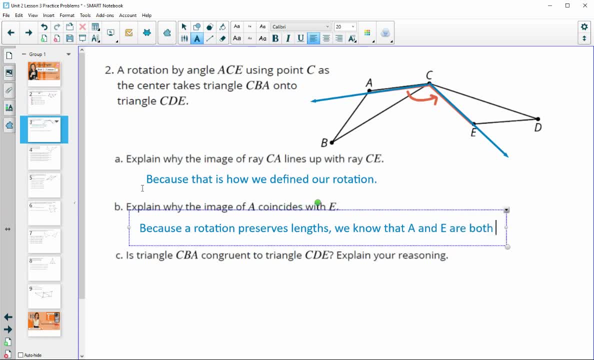 terminated. So because rotation preserves length, we know that A and E are both the same distance from point C. So since A is the same distance away from C and E is the same distance away from C, A will land directly on E, since they'll be on that. same ray. And then is triangle CE will land from the center of E to the central area and is disjixted from the center of A to B, which is the same distance between the two Officialastics. This plus, this plus, don't you perceive that these two are connected to each other? 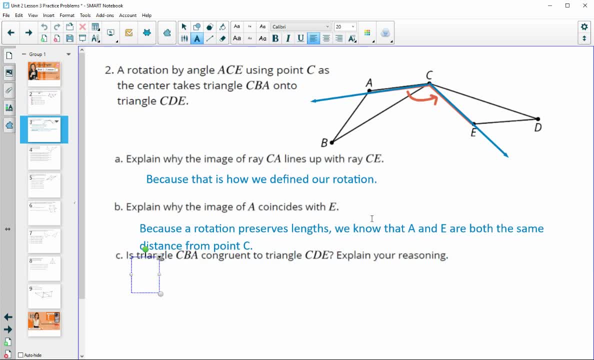 And right now, at table three, this points on the trapezoidal see, thatですか remains to be CBA congruent to triangle CDE. explain your reasoning. yes, because a rotation will preserve length and also we know that a will coincide with e, B will. 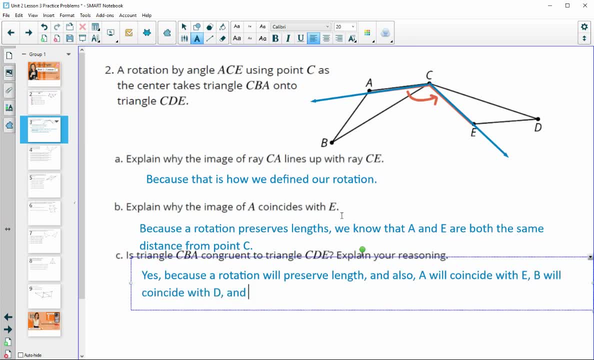 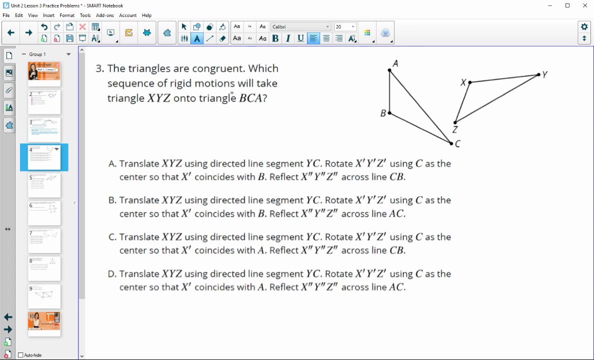 coincide with D and C is the same in both. so all three vertices are just gonna call it lined up. all right. then number three says these triangle CDE are congruent as opposed to triangle CDE. the triangle CDE has a, triangles are congruent. which sequence of rigid motions will take x, y, z on to a, b, c? 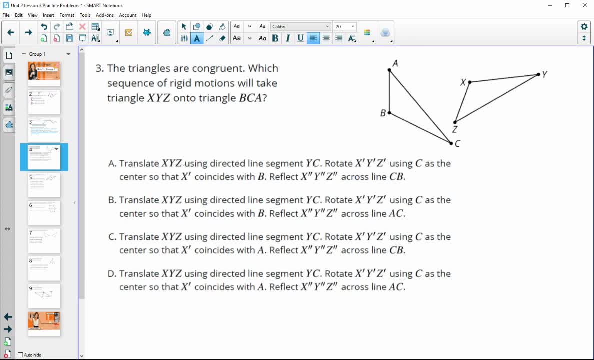 so the first one says: translate x, y, z using directed line segment y, c. okay, so it's going to take y and bring it to c. which are, though? do those um? are those corresponding is what we want to check out. so y to c is corresponding, so we want those two to coincide, so that part's good. 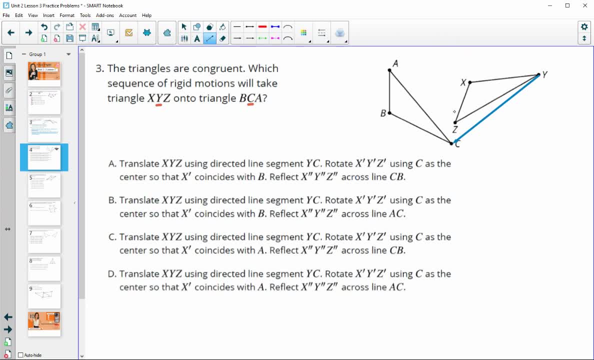 then it and let's see, let me actually draw this um triangle here so we can move it. so then this would move here. so now we've got y on c and then it says, using c as the center- okay, which is good, because that's the one we have marked up um rotate this new orange triangle. so 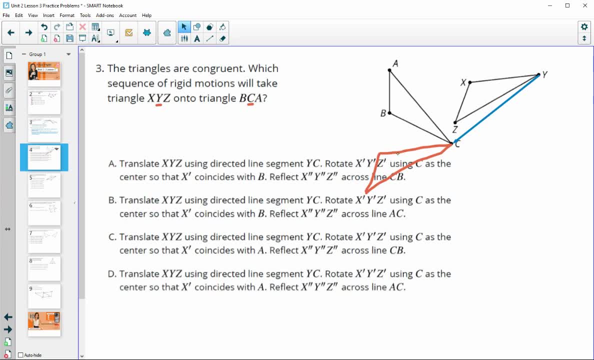 that x- which, if you remember, is right here, so here's x, so here's x. prime- coincides with b. so now they're saying: rotate this so that this coincides here. okay, which is good, that's what we want. so we want x to land on b, and so let's do that. 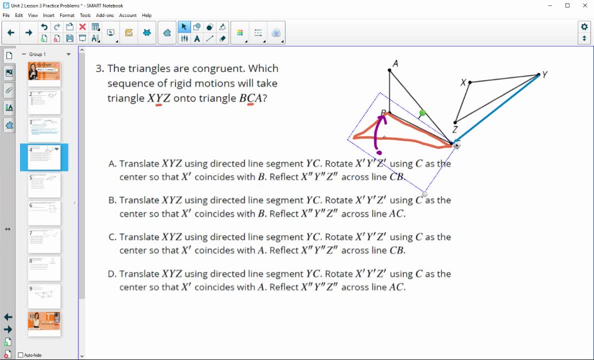 so that x lands on b. and then it says: now reflect this new triangle across the line c b. and here's c b reflecting it over. we'll put um z onto a. so this first one is actually the correct um sequence of rigid motions. so that was good um, if you're like me and you like it makes you nervous. 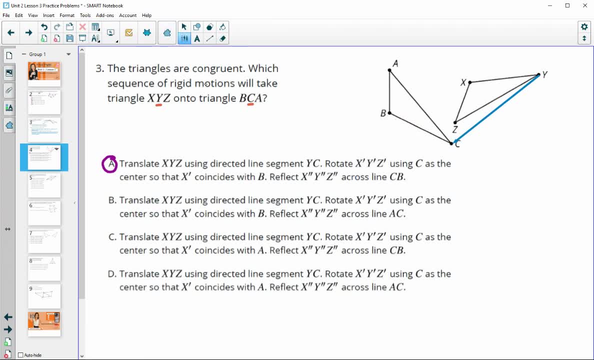 when the first one is the correct answer, you can look at the others to see where it goes wrong. so the first part here translate using directed line segment y: c is the same. so we kind of see the first same sentence in each one. so i'll leave this blue here. 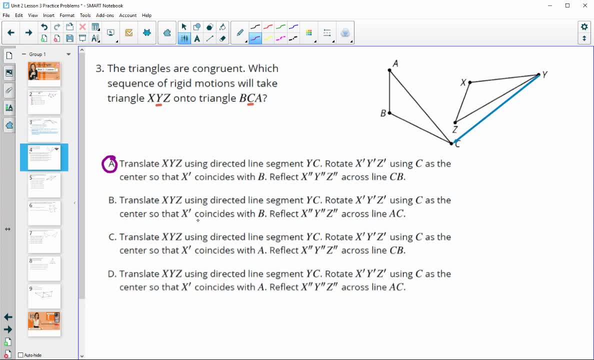 then it says rotate using c as the center, so that x coincides with b. that's the same. and then it says to reflect over line a, c, and we saw that that was incorrect, because we saw that the triangle was here. so we wanted to reflect over b, c, not a, c, um. so that's the issue. so here's the issue for this. 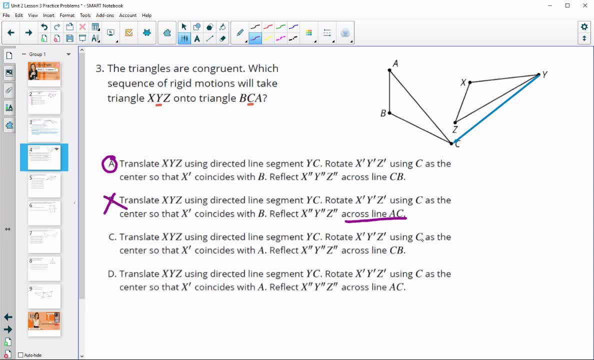 one to be untrue. this one says: rotates um using c as the center, so that x prime coincides with a. so now they're putting this angle on this one and those are not corresponding. so that would be bad. okay, so it's wrong here. and then this next one, or the last one. 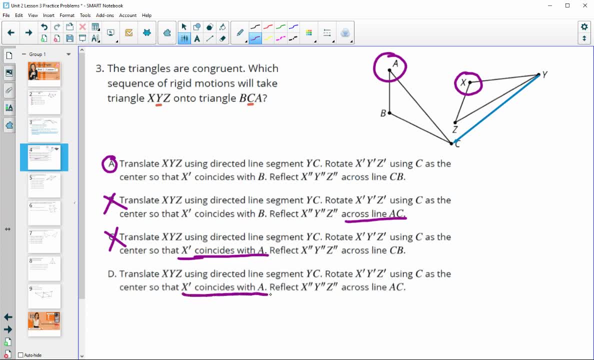 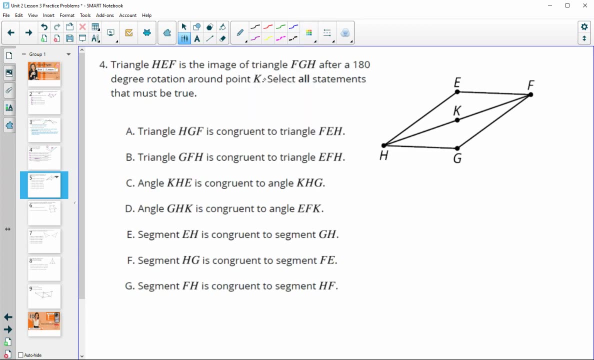 says rotate using c as the center, so that x prime coincides with a. so it says that again and those are not corresponding. so a was in fact the right one. number four triangle um is the image of f, g, h after 180 degree rotation around k. select all statements that are true. 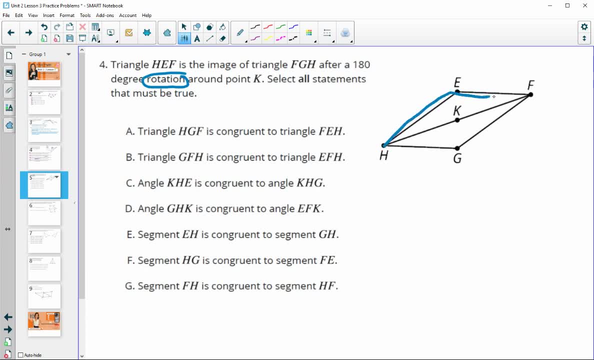 um, so we've got h, e, f, so this triangle here rotating around k. so let's just take a look at what that looks like to rotate here. so remember it looks like this: so we've got this h on top rotating to f. on the bottom, a e rotating to g. 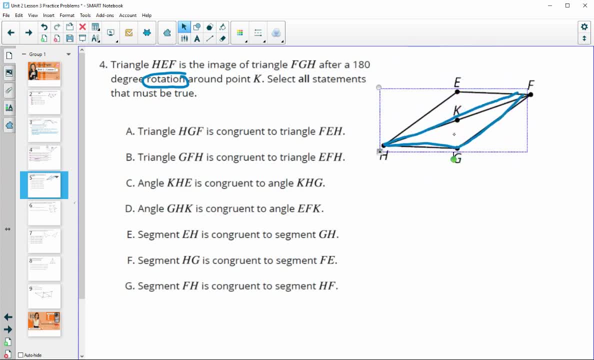 and then the f on top rotating to h on the bottom. so that kind of helps you remember what a rotation does. all right, so triangle, um h g f. so h g f is congruent to f e h. so let's um. so h g f- remember we got to look at the um order of the statement- is congruent to f e h, which is good. 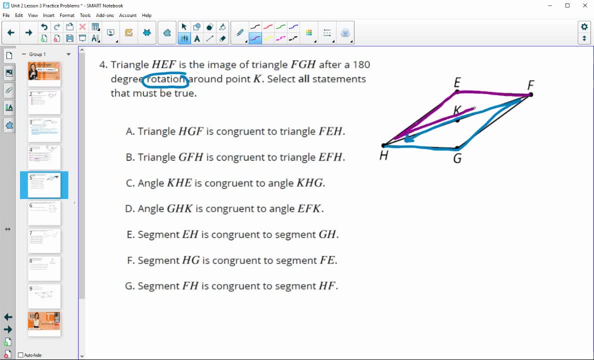 because then it goes f e, h here. so it's putting the blue h to the purple f, blue g to the purple e and then blue f to the purple h. so this is good triangle um g, f, h. so here's g f h is congruent to triangle. 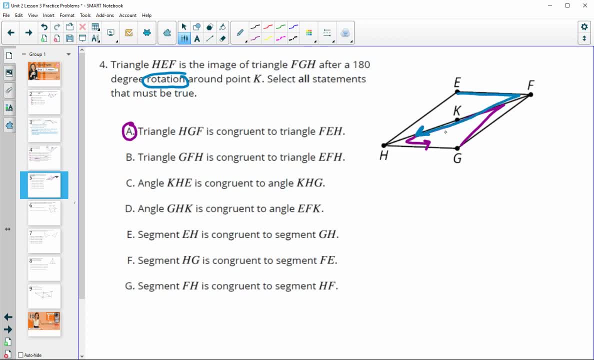 e, f, h, and that's bad because it's putting purple f with blue f and those two angles are not the same. remember it had to rotate. so this one's bad. um angle k, h, e, K, h, e, k, h, e. so angle k, h, e. so circled ein ist or a vor short. and then two angles: soään Io, angelo e angella wkw-nI existential. it's congruent to triangle e, f, h. and then two angles are not the same. remember it had to rotate, so this one's bad. 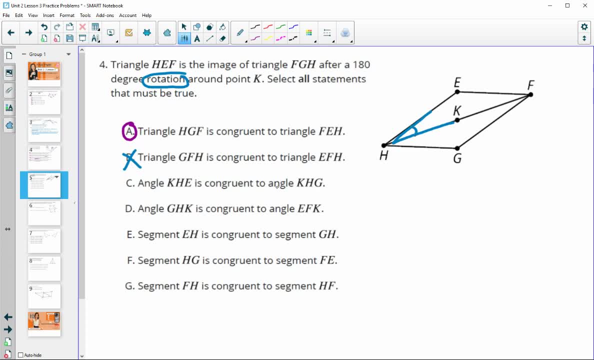 KHE. So this angle here is congruent to KHG, So KHG. So are those two angles congruent, And that's false. That happens in a reflection but not a rotation Angle. GHK is this one. Is that congruent to EFK? So EFK is here and that's true. 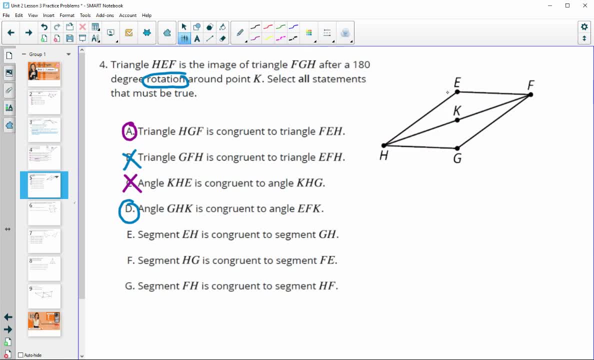 Segment EH is congruent to segment GH. Those two are not necessarily congruent. Again, that would happen in a reflection, but not in a rotation. HG is congruent to FH. FE, that is true. It'll rotate up onto that one. 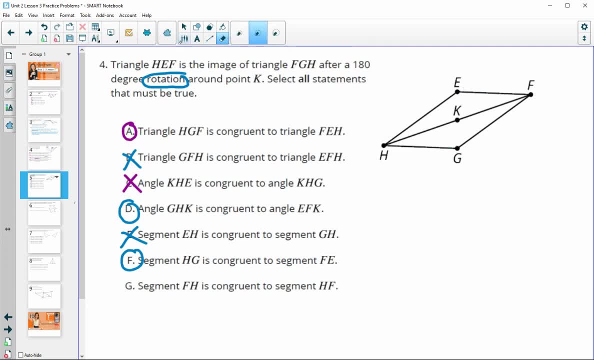 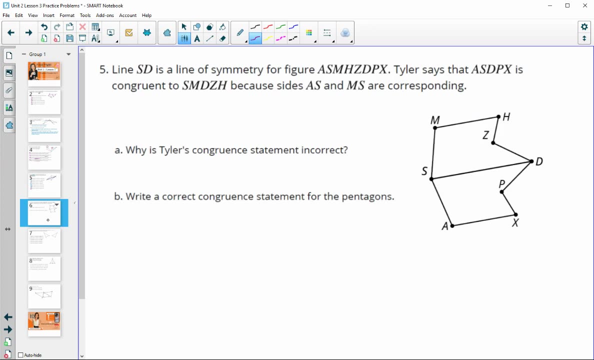 And then FH is congruent to HF, and that's true because those are the exact same segment, so they'd have to be the same Number. five line, SD, is the line of symmetry for this figure. Tyler says that Pentagon ASDPX is congruent to SMDZH because AS and MS are corresponding. So let's take a look at. 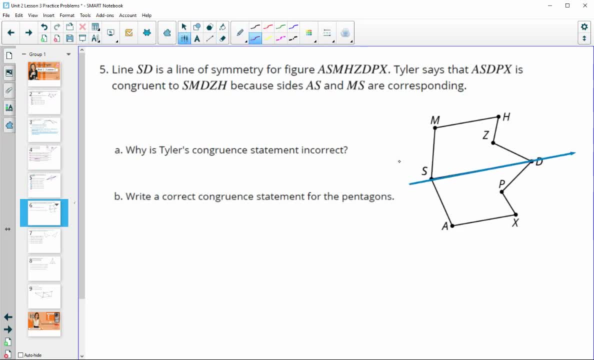 this. So here's our line of symmetry. and his order says AS, so his goes ASDPX, And then the other one goes SMDZH, And then it actually cuts across, so it goes SMDZH, So that one doesn't even follow the correct order. 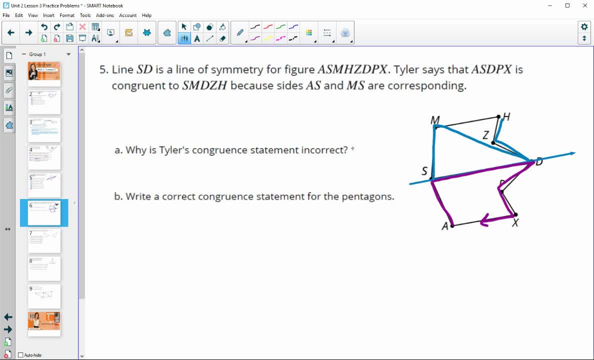 so that's one of the reasons it could be incorrect. The other is that this one started at A, so here was the first letter, and then went to S, So it went A to S And then, in this blue shape, it went. 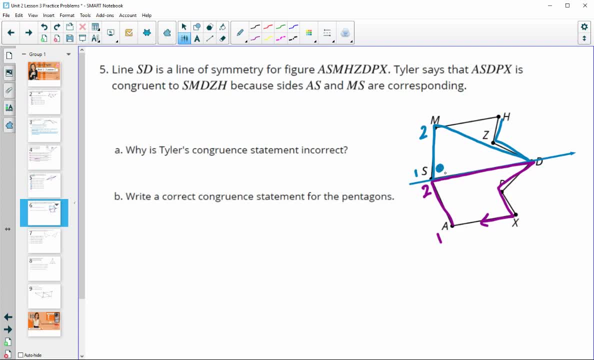 S to M And this angle does not match this angle. So A needed to match with M. So, even though A, S and SM are corresponding segments, angle A and angle S are not corresponding angles And both sides and angles need to match in the congruence statement. 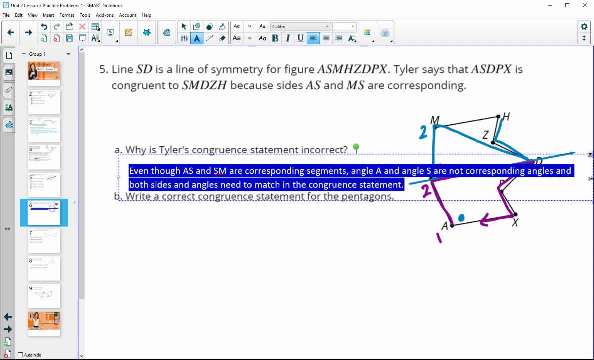 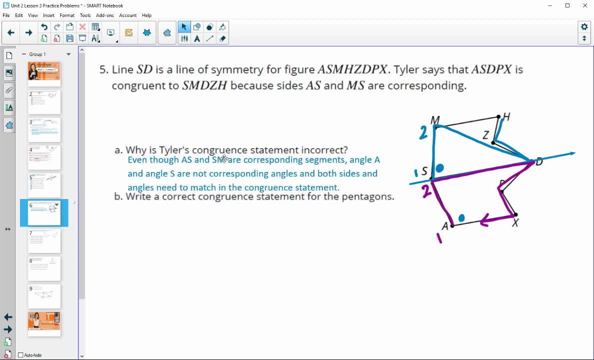 And again, the one was kind of cut across the shape too, so you know that the second one was not a good statement or not a good order. Anyways, I'm just going to put this up here, All right, and then write an actual congruence statement. 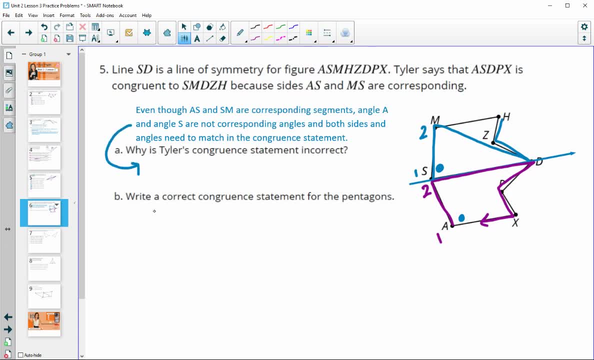 For them that works, And so I'm just going to start with this same first one that he did. A S D P X is congruent to, And so A went with M. So this is going to start M. 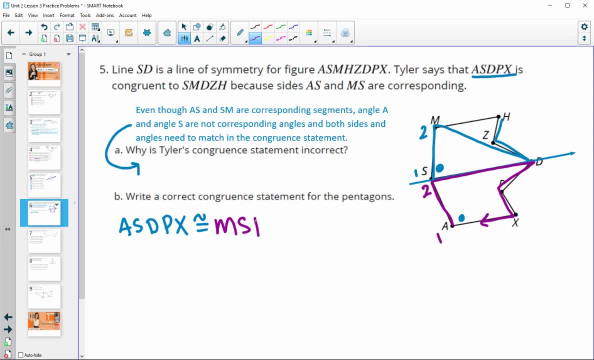 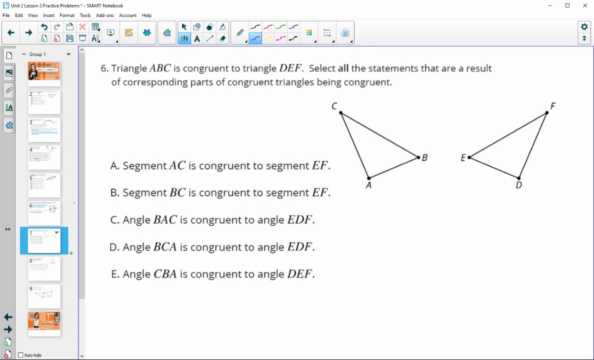 and then S to S, D to D and then P to Z and X to H. Number six triangle ABC is congruent to DEF. Select all statements that are a result of corresponding parts of congruent triangles being congruent, So you can just go by these. 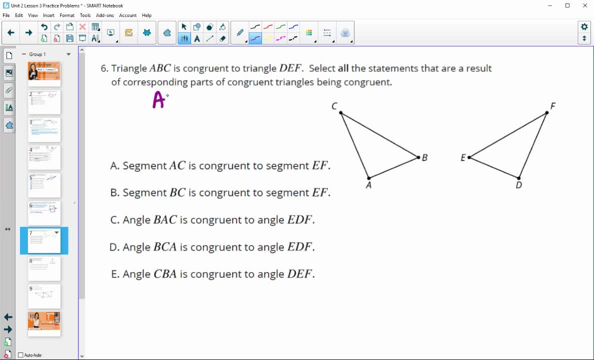 two statements. You can go by A, B, C and just compare the order DEF. So I like to kind of write them on top of each other sometimes to compare. You can also mark up the order DEF. So you can mark up the angles here. So A goes with D, B goes with E and then C goes with F. 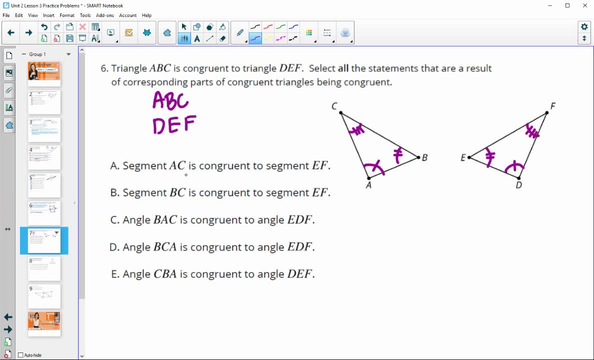 And that'll kind of help you look at it too. So AC is congruent to EF. So AC is the first and last. So it should go with DF, not EF. You can look here too. So AC goes with one and three, EF goes with two and connects angle two. 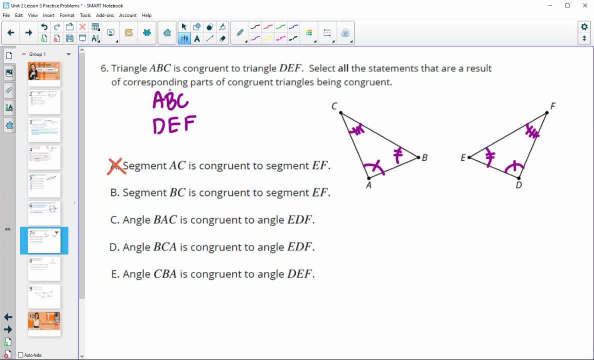 to three. So that's not going to be good. Segment BC: So that's these last two letters here- is congruent to EF- the last two letters there. So those are corresponding, So that's good. Angle BAC: is this one congruent to EDF? this one, That is true, You can look at the middle. 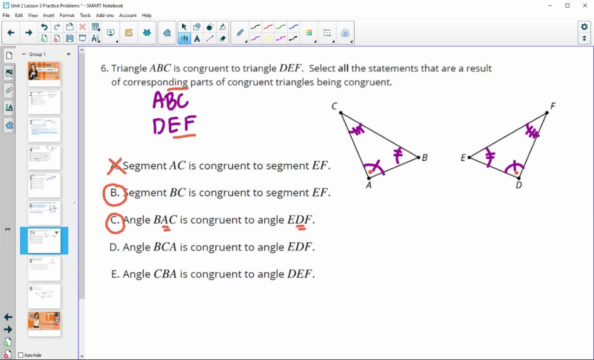 the letter for the vertex. So angle A to angle D and C in the statement. So in this one, B, C, A is this one, E, D, F is this one. Those are not corresponding, So that would be false. 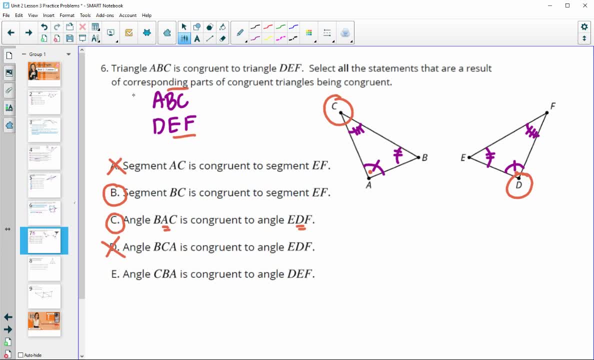 And then CBA. So CBA, is this one congruent to D? So that's true. You can look here too, So that's good Angle. BAC: is this one congruent to DEF? So this one, And that is true. 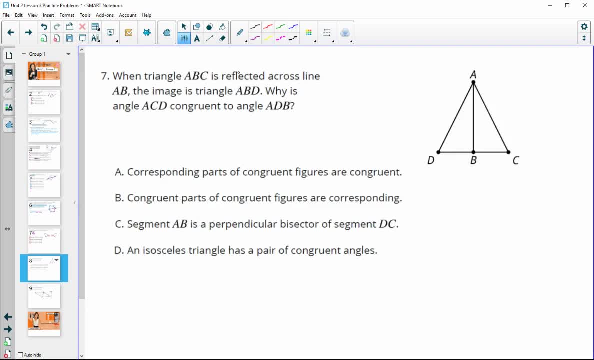 Number seven. when triangle ABC is reflected across the line AB, the image is ABD, Y is angle ACD. So this angle congruent to angle ADB. So when we reflect this over those are corresponding parts And we know reflection gives us congruent triangles.